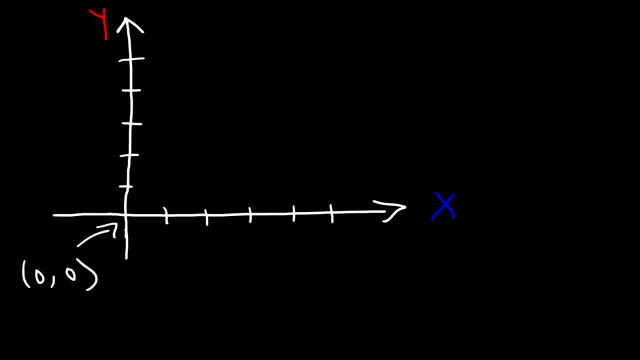 So this is a coordinate system. Now let's say, if we want to plot point A, and point A is located at 2, 3.. The first number is a coordinate system, the x-coordinate, and the second number is the y-coordinate. So to plot it we need to. 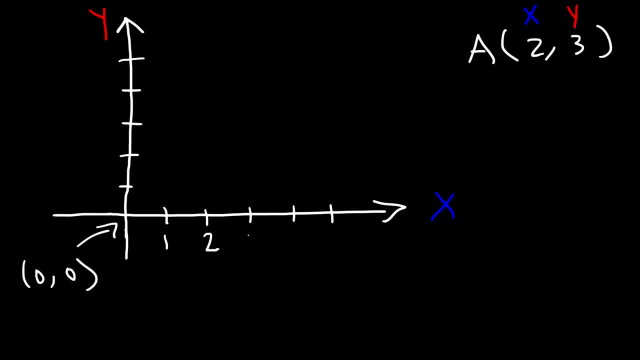 locate 2 on the x-axis and then we need to locate 3 on the y-axis. So here's 2 on the x-axis. in history, Therefore, point A is going to be at that location. So here it is. Now let's try a few more examples. Go ahead and plot point B and let's say it's located. 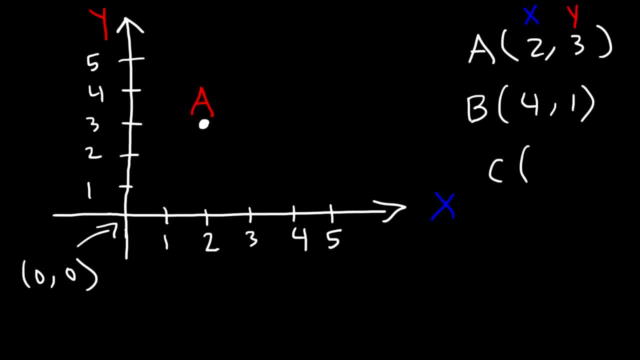 at 4, 1 and plot point C, which is located at 3, 2.. So the x-value is located at 3, 2.. So the x-value is located at 3, 2.. The y-value is 4 and the y-value is 1.. 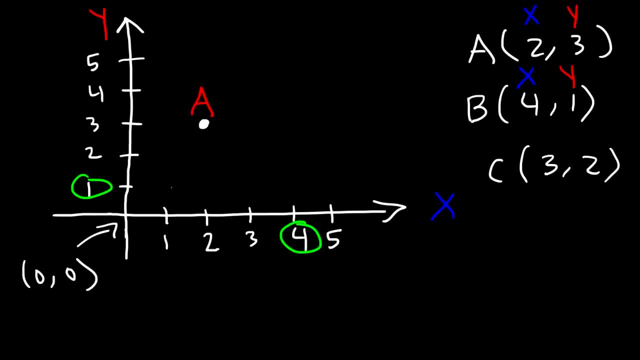 So here we have an x-value of 4 and a y-value of 1.. Therefore, they should meet at that point. So this is going to be point B. Now, to plot point C, we need to locate an x-value of 3 and a y-value of 2, which corresponds. 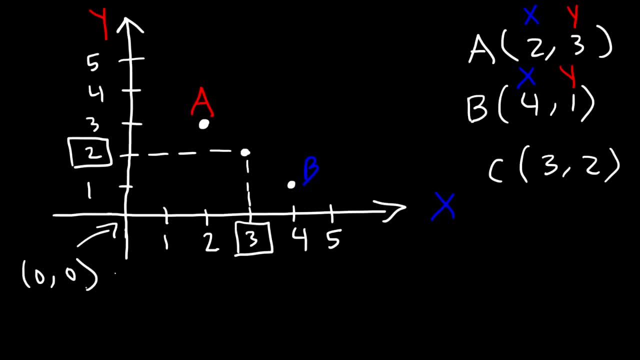 to this point. That's where they intersect, And so that's going to be point C, And so that's how you can plot a set of ordered pairs on a graph or on a coordinate plane, And these are ordered pairs, by the way. 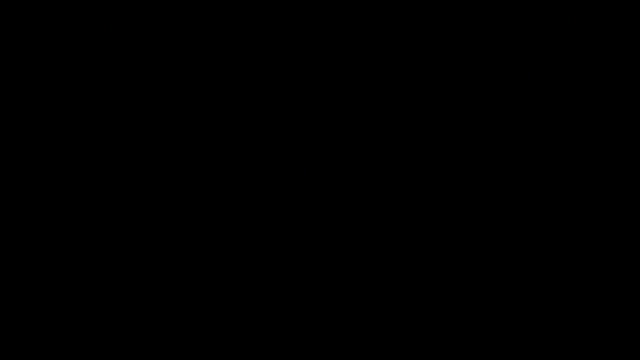 You have an x-coordinate and a y-coordinate. Now let's try some more examples. Go ahead and plot the following points: 3, 4, negative 2, 3, negative, 4, negative 2, and 3, negative 3.. 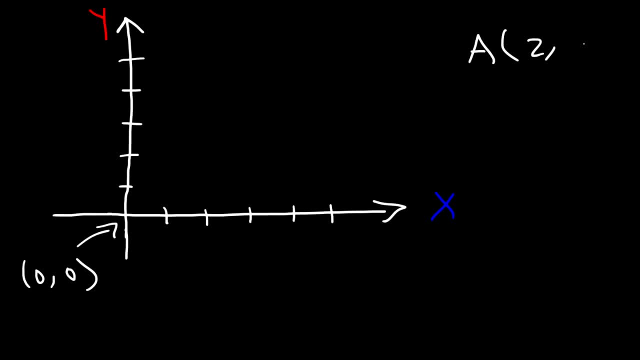 This point is known as the origin, And it's 0, 0.. the x-coordinate, and the second number is the y-coordinate. so to plot it, we need to locate 2 on the x-axis and then we need to locate 3 on the y-axis. so 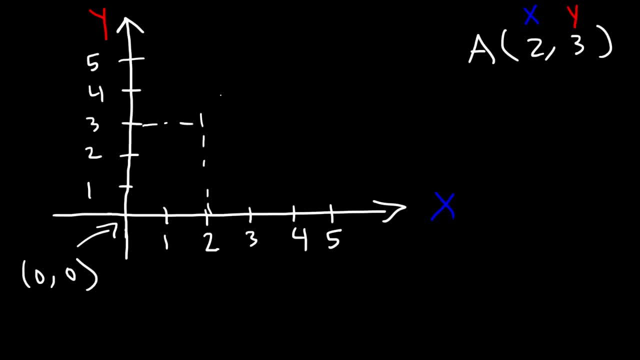 here's 2 on the x-axis in history. therefore, point a is going to be at that location. so here it is. now let's try a few more examples. go ahead and plot point B, and let's say it's located at 4: 1, and plot point C, which is located at. 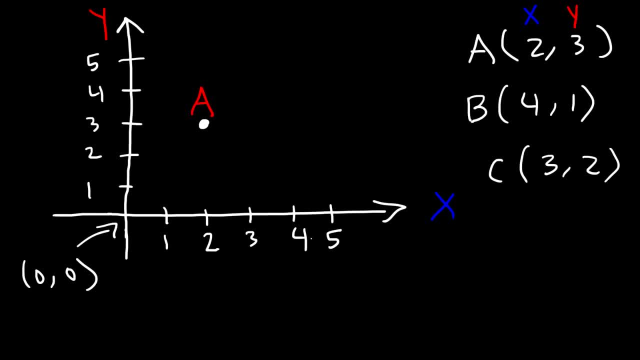 3, 2, so the X value is 4 and the Y value is 1. so here we have an X value of 4 and the Y value of 1, therefore they should meet at that point. so this is going to be point B. now to plot point C, we need to 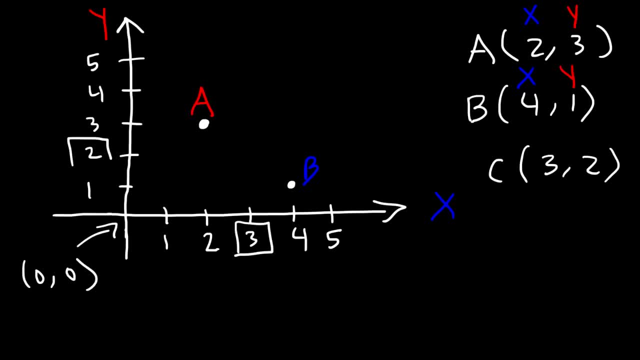 locate an X value of 3 and a Y value of 2, which corresponds to this point. that's where they intersect, and so that's going to be point C, and so that's how you can plot a set of ordered pairs on a graph or on a coordinate plane, and these are: 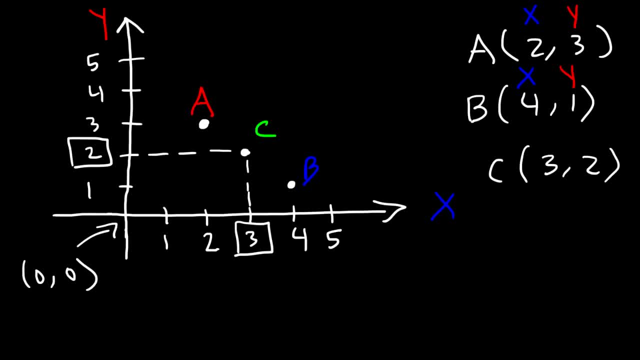 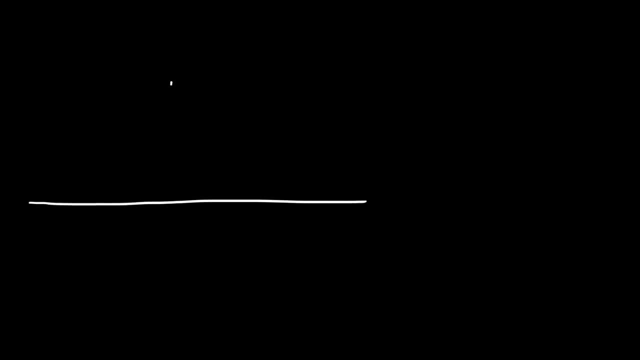 ordered pairs. by the way, you have an x-coordinate and a y-coordinate. now let's try some more examples. go ahead and plot the following points: 3 comma, 4 negative, 2, 3 negative, 4 negative 2 and 3 negative 3. so feel free to pause the. 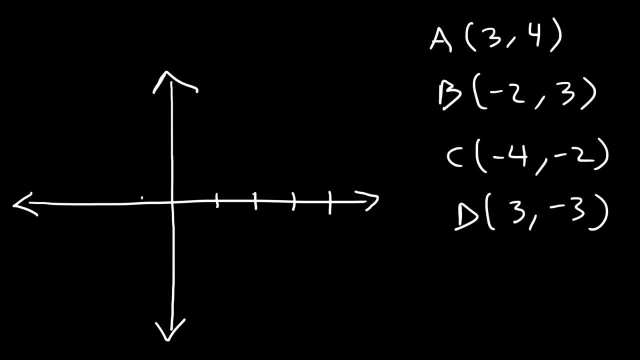 video, as you are plot those points. so this is positive 4, and over here we're going to have negative 4. so let's start with 3 comma 4. so here's an X value of 3, here's a Y value of 4. they're going to meet at that. 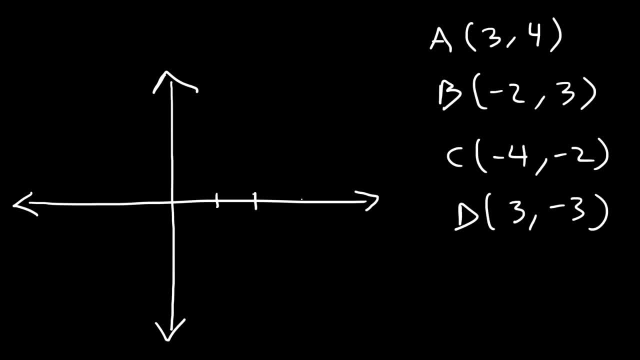 So feel free to pause the video as you plot those points And you can see that the x-value is located at 3,, 2, and a y-value of 1. So this is positive 4.. And over here we're going to have negative 4.. 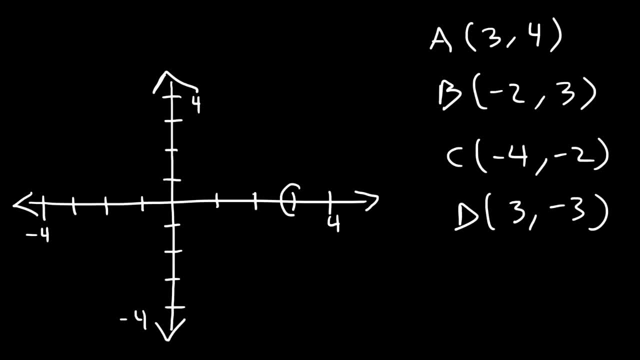 So let's start with 3, 4.. So here's an x-value of 3.. Here's a y-value of 4.. They're going to meet at that point. So right, here is 3, 4.. It's in the first quadrant. 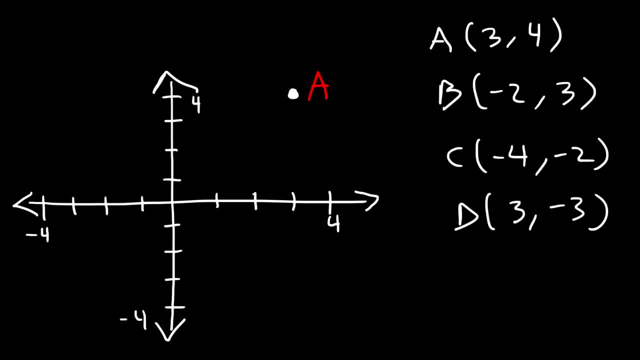 And that's going to be point A. Next let's plot point B, which is at negative 2, 3.. Point B is in quadrant 2.. And then let's plot point C, which is at negative 4, negative 2.. 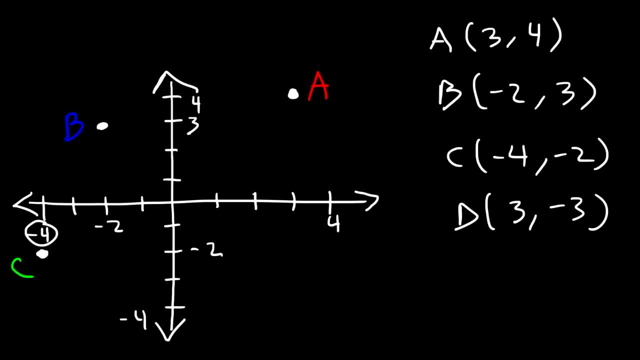 Point C is in quadrant 3.. And after that we have 3, negative 3,, which is right here, And that's in quadrant 4.. And so now you know how to graph ordered pairs on a coordinate plate. Now the next thing that you need to be able to do is to identify the points that are found on a coordinate plate. 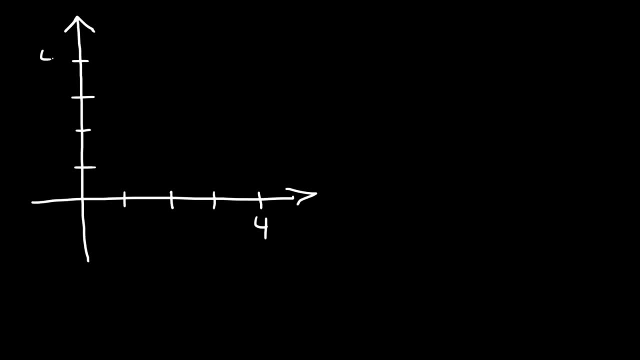 So I'm going to give you three points And I want you to write the coordinates of these three points. So here's the first one. We're going to call that point A. And here's the second one. Let's call this point C. 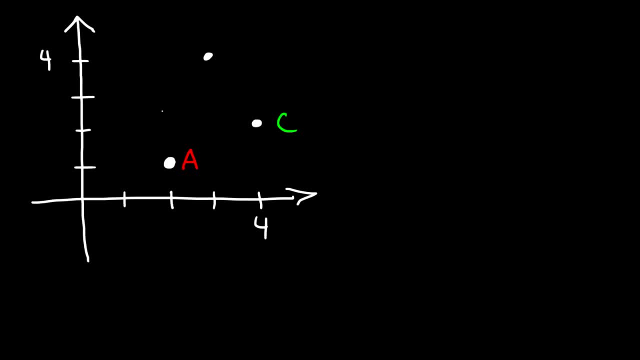 And the last one is going to be over here, Let's call it point B. So go ahead and find the x and y coordinates of those points. So let's start with the first ordered pair, point A. Point A has an x-value of 2 and a y-value of 2.. 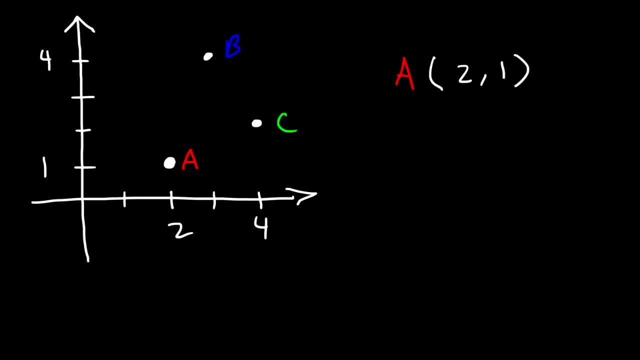 And it has an y-value of 1.. So it's 2, 1.. Next we have point B. Point B has an x-value of 3. And it has a y-value of 4. So it's 3, 4.. 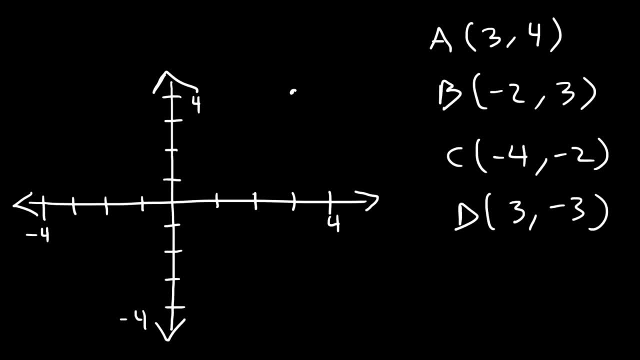 point. so right, here is 3 comma 4. it's in the first quadrant and that's going to be point A. next let's plot point B, which is that negative 2 comma 3. point B is in quadrant 2, and then let's plot point C, which is that negative 4, negative 2. point C is in. 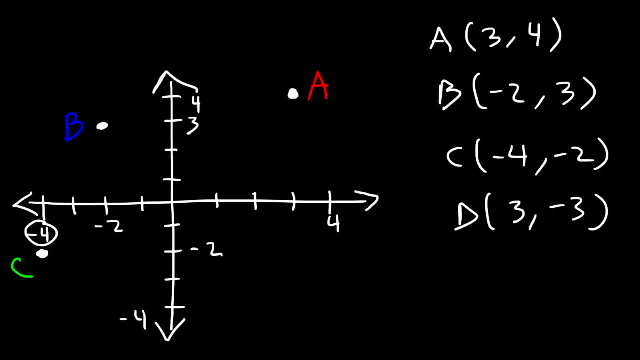 quadrant 3, and after that we have 3 comma negative 3, which is right here, and that's in quadrant 4, and so now you know how to graph ordered pairs on a coordinate plate. now the next thing that you need to be able to do is to: 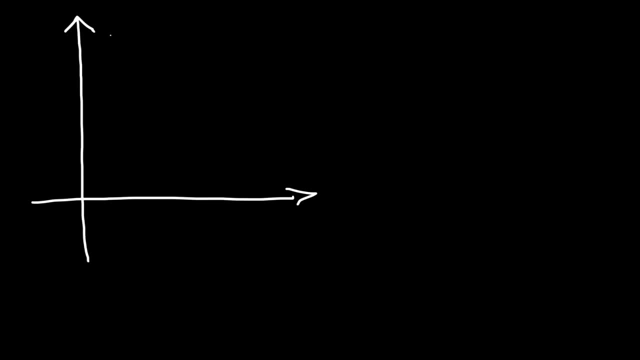 identify the points that are found on a coordinate plane. so I'm going to give you three points and I want you to write the coordinates of these three points. so here's the first one. we're going to call that point A. and here's the second one. let's call this point C. and the last one is going to: 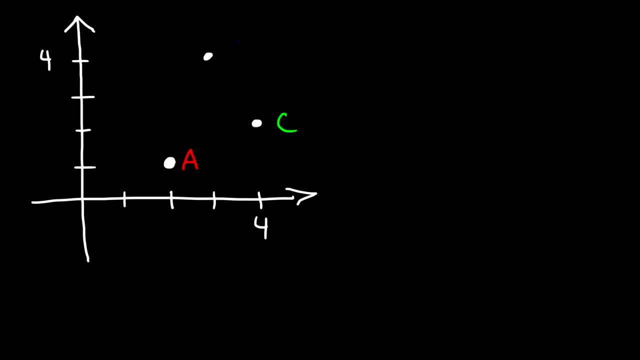 be over here. let's call it point B. so go ahead and find the X and Y coordinates of those points. so let's start with the first ordered pair, point A. point A has an X value of 2 and the Y value of 1, so it's 2 comma 1. 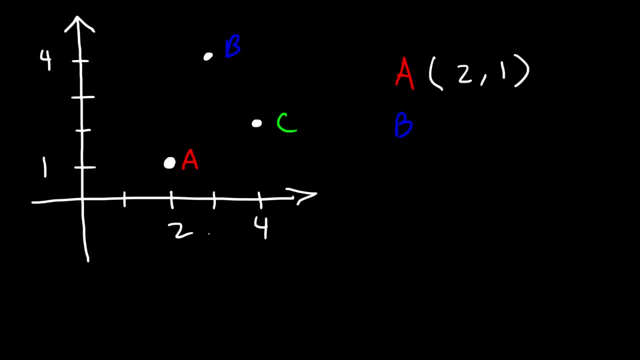 next we have point B. Point B has an x value of 3 and it has a y value of 4.. So it's 3, 4.. Next let's move on to point C, which has an x value of 4 and it has a y value of 2.. And so that's it. That's how you can. 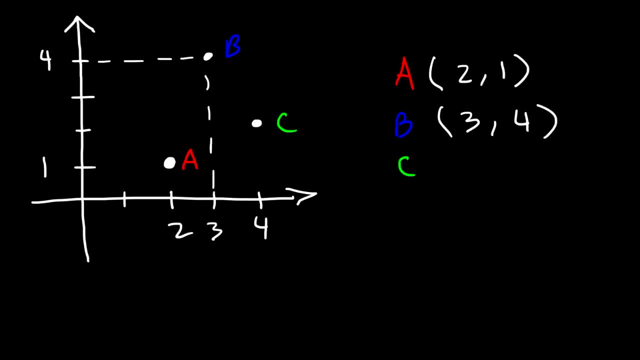 Next, let's move on to point C, which has an x-value of 4. And it has a y-value of 2. And it has a y-value of 2.. And so that's it. That's how you can identify an ordered pair if you're given a graph. 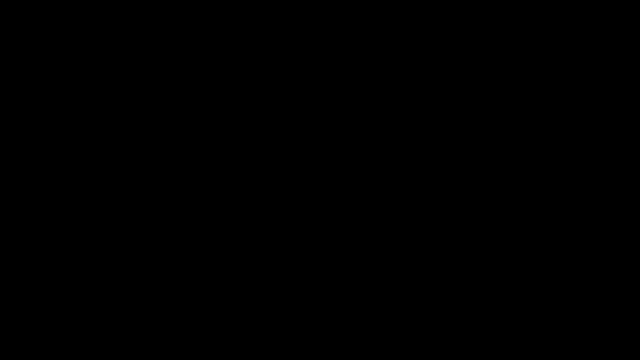 Now the next thing that we need to talk about is a relation. A relation is basically a set of ordered pairs. So let's say, if we have the ordered pairs negative, 2, 3, 1, 2, 1, 2,. 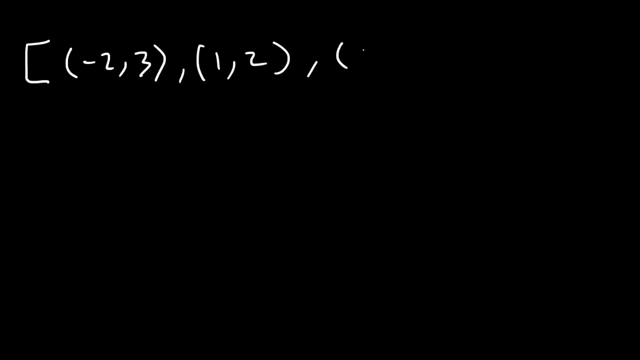 2, 5, and 4, 7.. So all four of those ordered pairs combined comprises a relation. Now you need to be able to determine the domain and the range. The domain of the relation is basically the set of all the x-values. 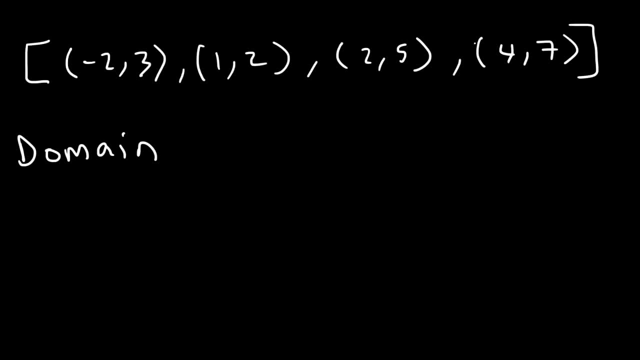 or all of the x-coordinates. So the x-coordinates that we have are negative 2,, 1,, 2, and 4.. So therefore, that's going to represent the domain. So it's negative: 2,, 1,, 2, and 4.. 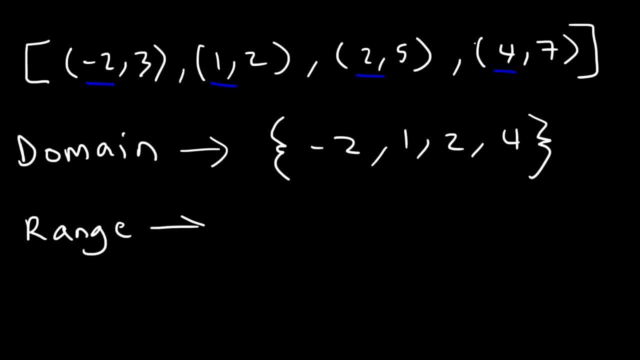 Now, what about the range? The range represents all of the y-coordinates, The y-coordinates being 3,, 2,, 5, and 7.. And now let's put the y-values in ascending order. So the lowest value is 2, and then we have 3,, 5, and 7.. 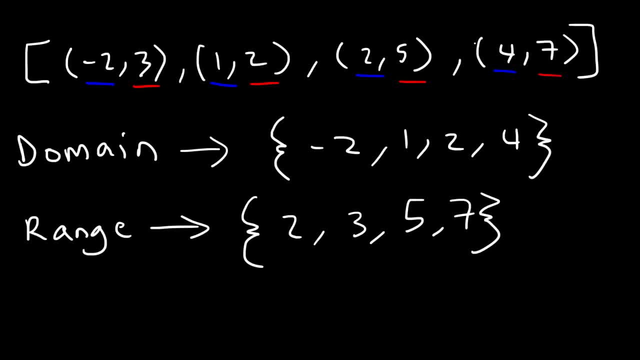 So that's the range which correlates to all of the y-values. Now, if you don't want to put it in ascendant order, you can write it the same way, exactly as you saw it. So, for example, you could write it as 3,, 2,, 5,, 7, and 8.. 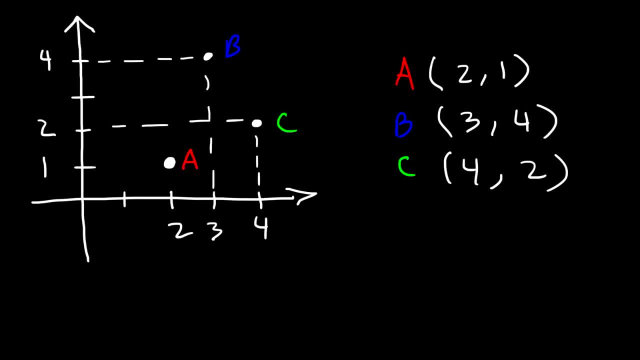 identify an ordered pair if you're given a graph. Now the next thing that we need to talk about is a relation. A relation is basically a set of ordered pairs. So let's say, if we have the ordered pairs negative, 2, 3, 1, 2,, 2, 5, and 4, 7.. 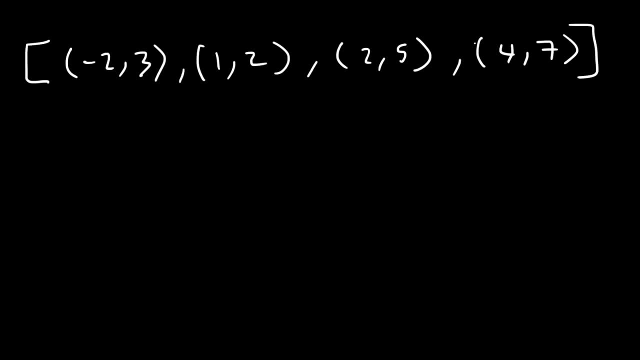 So all four of those ordered pairs combined comprises a relation. Now you need to be able to determine the domain and the range. The domain of the relation is basically the set of all the x values or all of the x coordinates. So the x coordinates that we have are negative: 2,, 1,, 2, and 4.. 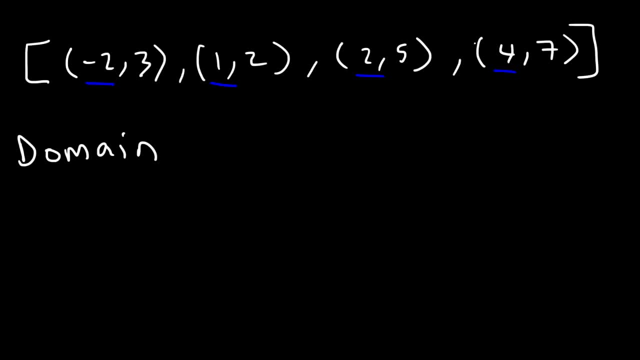 So, therefore, that's going to represent the domain. So it's negative: 2,, 1,, 2, and 4.. Now what about the range? The range represents all of the y coordinates, The y coordinates being 3,, 2,, 5, and 7.. But now let's put the y values in ascending order. 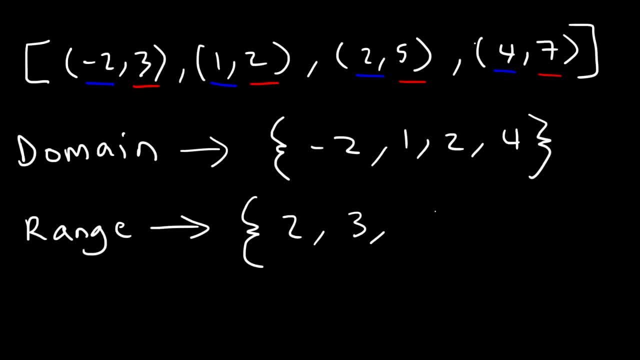 So the lowest value is 2,, and then we have 3,, 5, and 7.. So that's the range which correlates to all the y values. Now, if you don't want to put it in ascending order, you can write it the same way. 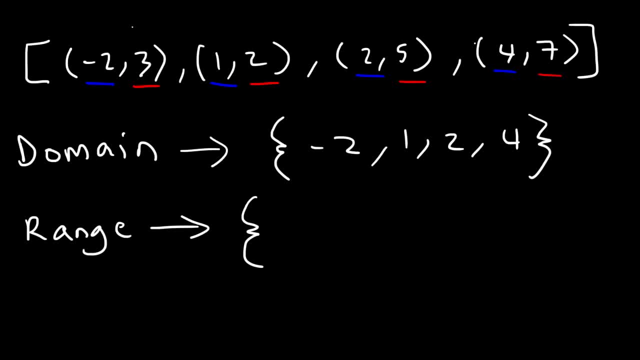 exactly as you saw it. So, for example, you could write it as 3,, 2,, 5, 7.. So you could write it the that way. if you want to. A relation can also be represented in the form of a table. So consider this table. with the following points, You can convert a table. 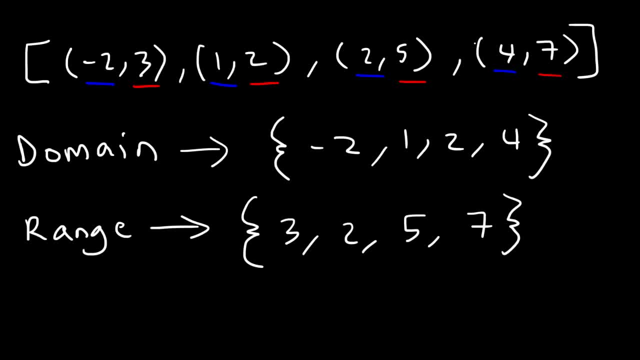 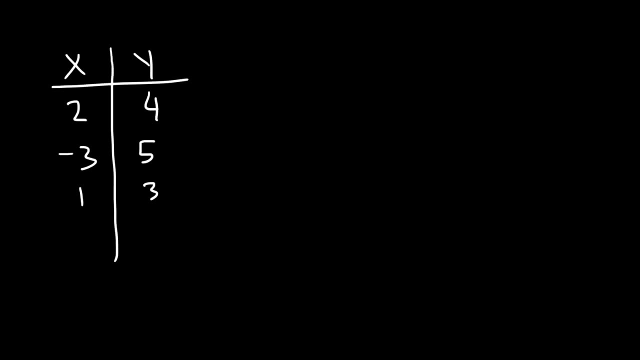 So you could write it that way if you want to. A relation can also be represented in the form of a table. So consider this table with the following points: You can convert a table into a set of ordered pairs. So the first ordered pair is 2, 4.. 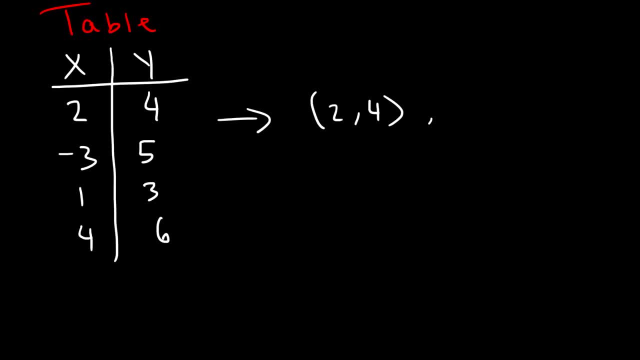 The second is negative: 3, 5.. The third is 1, 3.. And the fourth is 4, 6.. Now to find the domain which I'm going to use the letter D to represent the domain. the domain is just all of the x-values which we can see here. 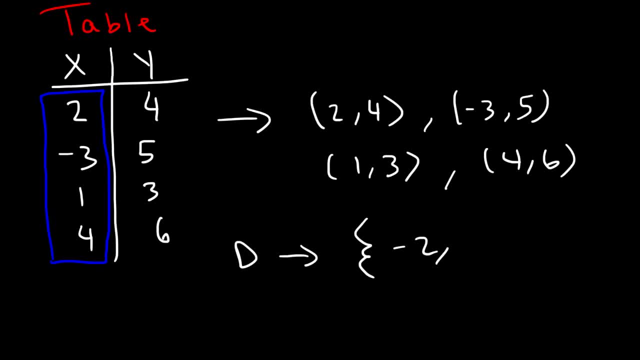 So it's going to be negative 2,. I mean not negative 2,, but rather positive 2.. And then negative 3,, 1, and 4.. So that's the domain. The range represents all of the y-coordinates. 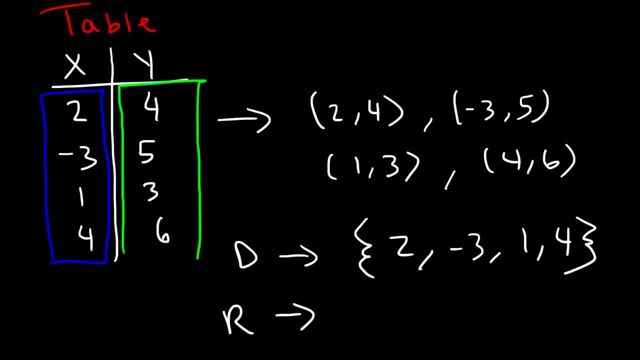 which we can clearly see it on the second column of the table, And that's going to be 4,, 5,, 3, and 6.. So that's how you can find the domain and range of a relation when it's expressed in the form of a table. 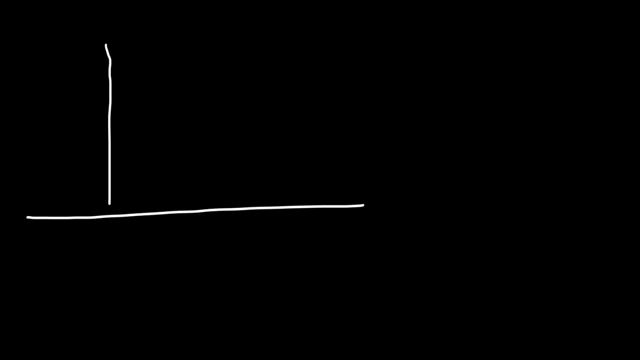 Now the last thing is: you need to find it if it's expressed in the form of a graph. So let's say, if we have this point, that's the first point, and here is the second point, and here's the third. 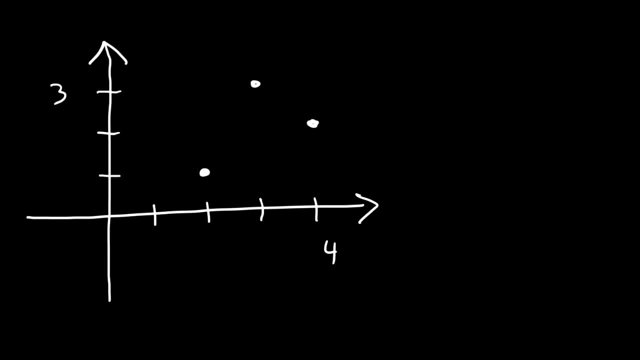 Go ahead and find the domain and range of this graph. So the domain is all of the x-values. We have an x-value at 2,, 3, and 4.. This one's at 2,, this one's at 3, and that one's at 4.. 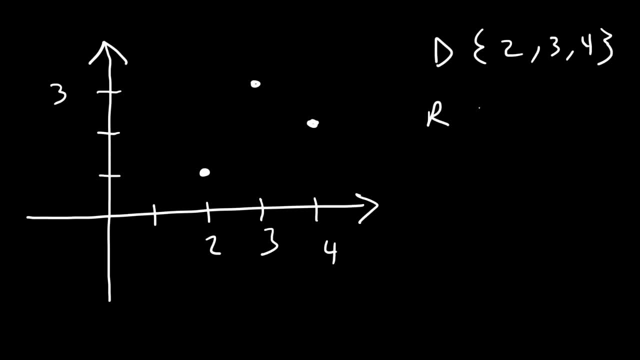 Now for the range. we need to write the y-values. So this point has a y-value of 1,, this one has a y-value of 2, and this one has a y-value of 3.. So the range is 1,, 2,, 3.. 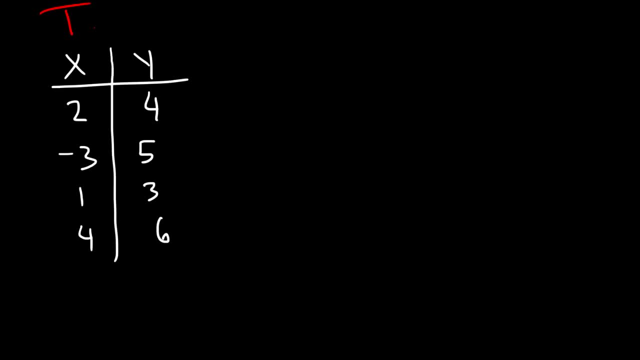 into a set of ordered pairs. So the first ordered pair is 2 comma 4.. The second is negative, 3 comma 5.. The third is 1 comma 3.. And the fourth is 4 comma 6.. Now to find. 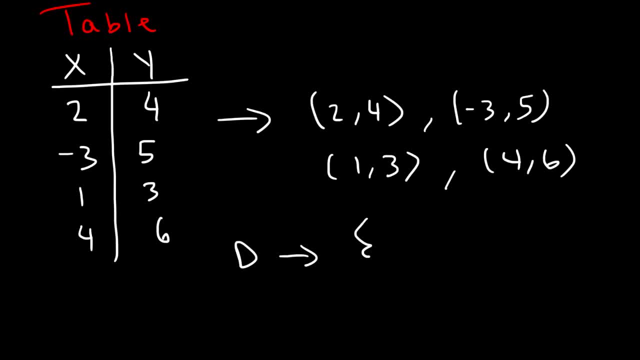 the domain which I'm going to use the letter D to represent the domain. The domain is just all of the x values which we could see here, So it's going to be negative 2, I mean not negative 2, but rather positive 2, and then negative 3,, 1, and 4.. So that's the domain, The range. 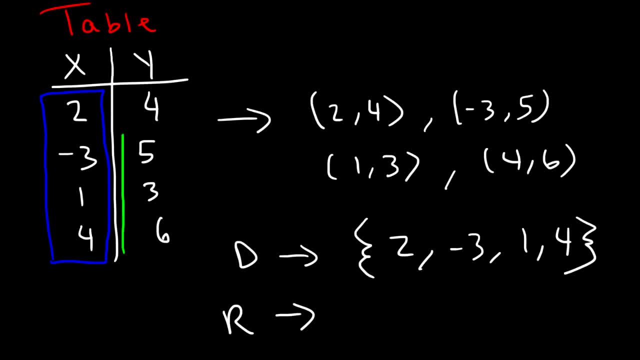 represents all of the y-coordinates which we can clearly see it on the second column of the table, And that's going to be 4, 5,, 3, and 6.. So that's how you can find the domain and range of a relation when it's. 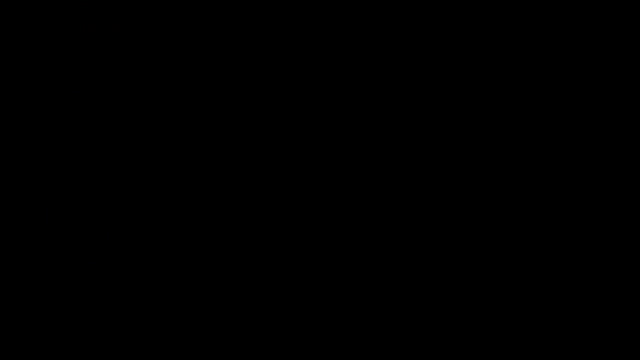 expressed in the form of a table. Now, the last thing is, you need to find it if it's expressed in the form of a graph. So let's say, if we have this point, that's the first point and this is the second point. 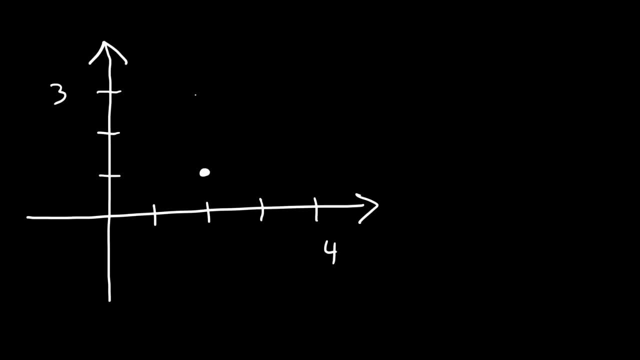 and this is the third point, and this is the fourth point, and this is the fifth point, and this is the fifth point, and this is the sixth point, and this is the last point. the first point, and here is the second point, and here's the third. go ahead and. 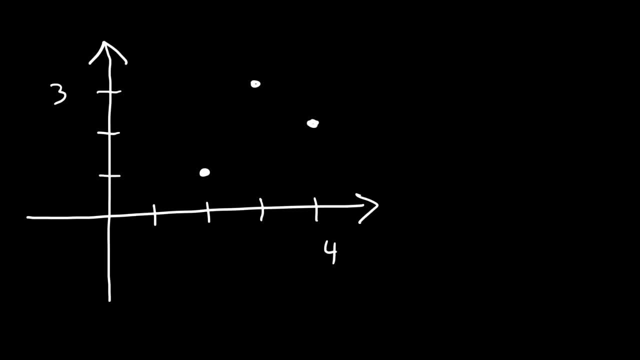 find the domain and range of this graph. so the domain is all of the X values. we have an X value at 2, 3 & 4, this one's at 2, this one's at 3 and that one's at 4. now for the range we need to. 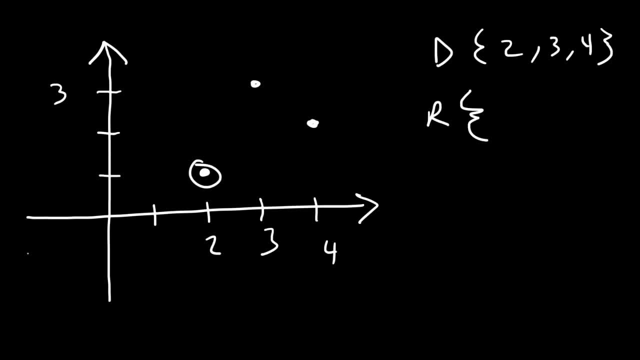 write the Y values. so this point has a Y value of 1, this one has a Y value of 2 and this one has a Y value of 3. so the range is 1, 2, 3, and so that's how you can easily determine the domain and range of a set of points, given the graph.